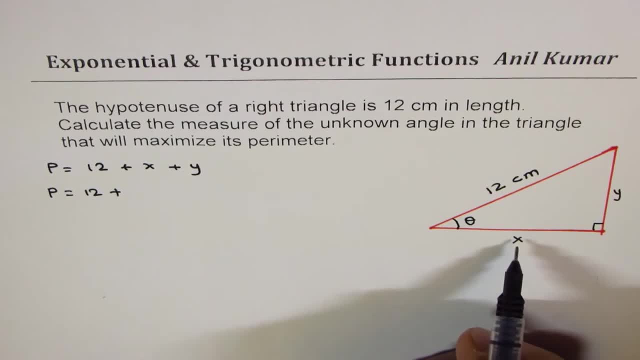 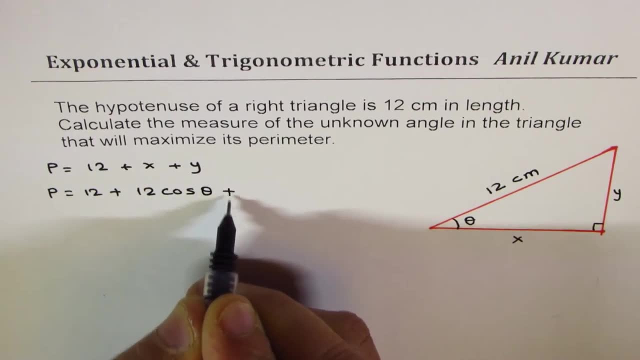 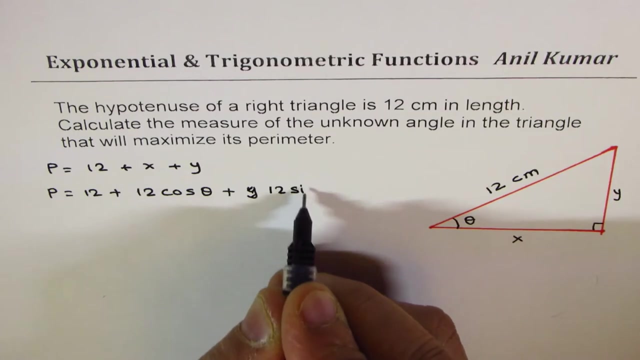 Now that is the adjacent side, which has to be smaller than hypotenuse. It becomes 12 cos of theta, plus y Will be equals to 12 sine of theta, right, So we'll replace that by 12 sine theta. 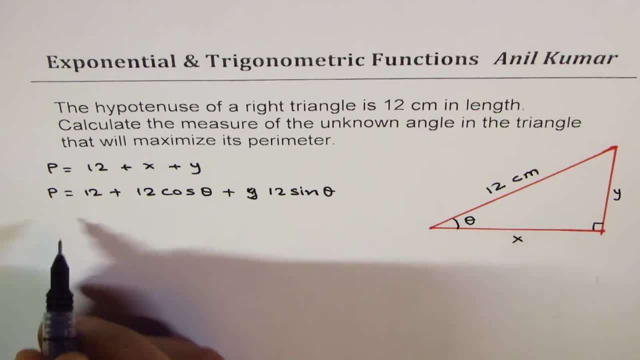 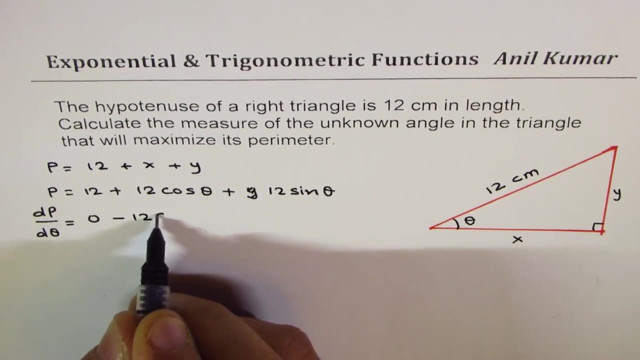 To maximize the perimeter, we'll find the derivative with respect to theta, That is, dP. d theta is equal to derivative of constant in 0 plus 12 cos. theta derivative is minus 12 sine theta And the derivative for plus 12 sine theta. 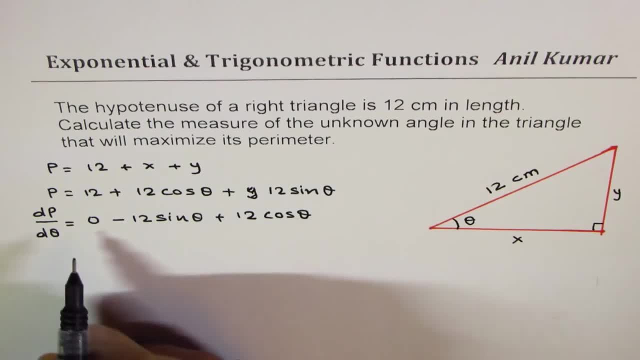 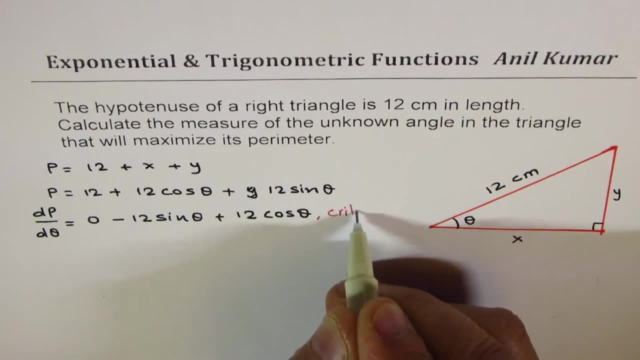 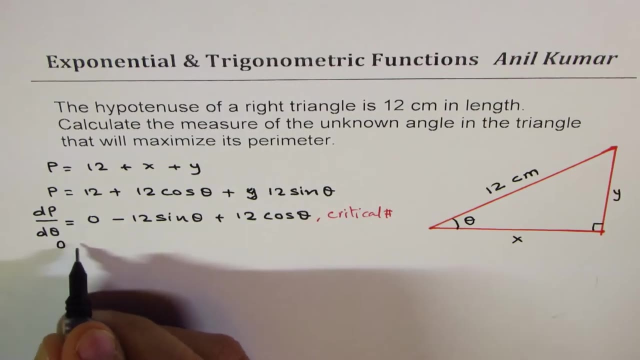 is 12 cos theta. ok, Quotient For a critical number. we have to equate this derivative to 0. So let's find the critical number first. So that means 0 is equal to: we have minus 12 sine theta, plus 12 cosine theta, bringing terms to the left. cancellation of 12 sine theta. 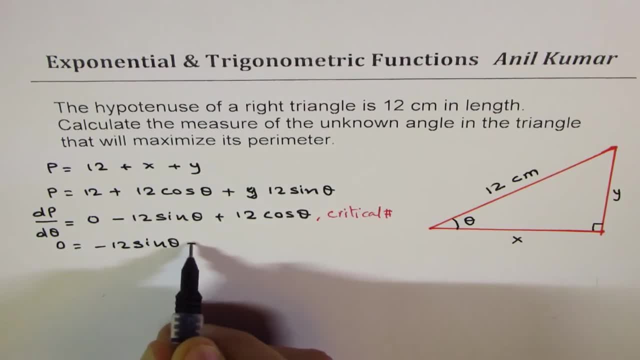 We can find the first けady get a tiny fringe. K Rs mean very kinds many radians and plus 12 cosine. theta Muniz means that determindan four and three into the math, that we can choose the terms that belong to s. 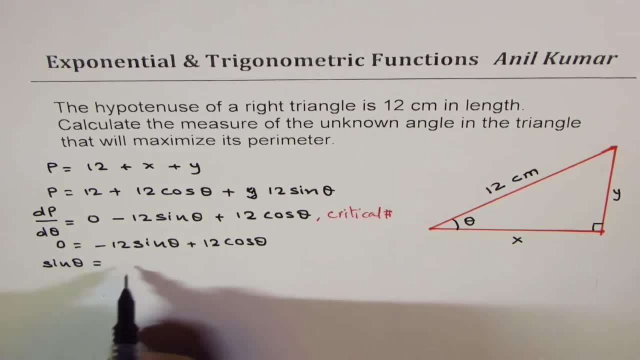 And the sum of all the correct values boundary along theير r kind. well, we get sine theta equals to cosine theta dividing. we get sine theta divided by cos theta equals to 1, which is tan theta equals to 1 and from here you can get theta as tan inverse. 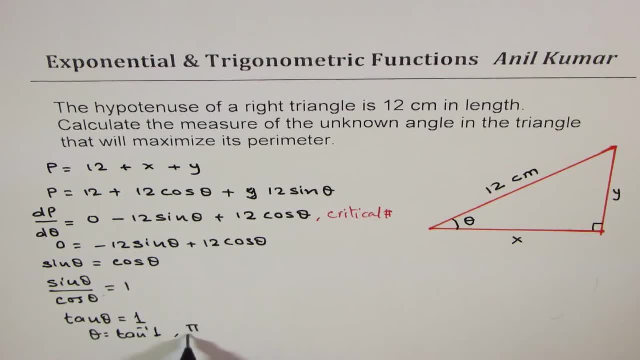 of 1, which is pi by 4, right? so you get pi by 4 as the option. now, whether it really gives you a maximum or a minimum, you can test it out by finding the second derivative of the given function, right? so let's find the second derivative. d2p d theta square equals to: 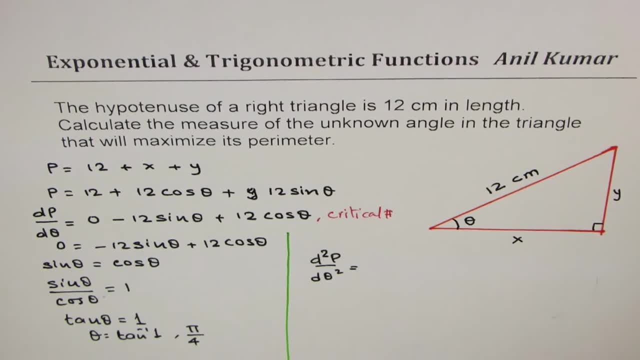 so when you do second derivative, we are using this particular equation: negative 12 cosine theta right and cos theta derivative is negative. we get negative 12 sine theta. now in this case, if i take negative 12 common, i'm left with cos theta plus sine theta as the result.